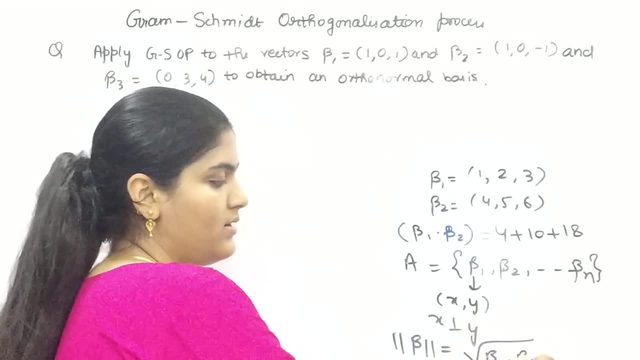 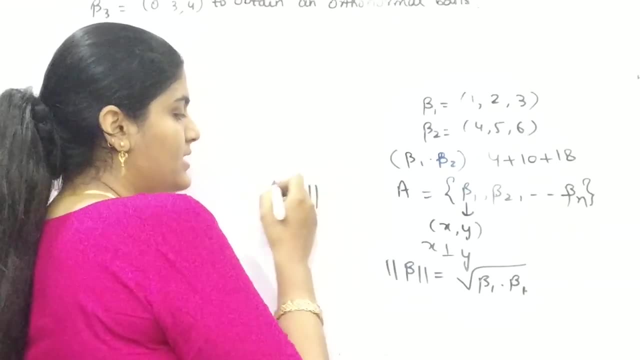 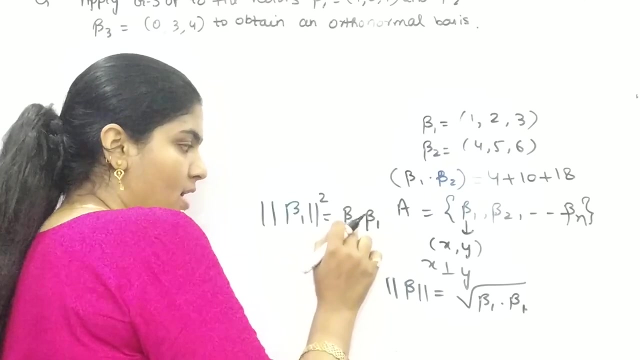 root of the inner product. So you have to multiply, take the root of the inner product of those. Why? Because, if you see, if you will take the square of this, then it will be beta 1 into beta 1.. Right, And which means you are multiplying them And 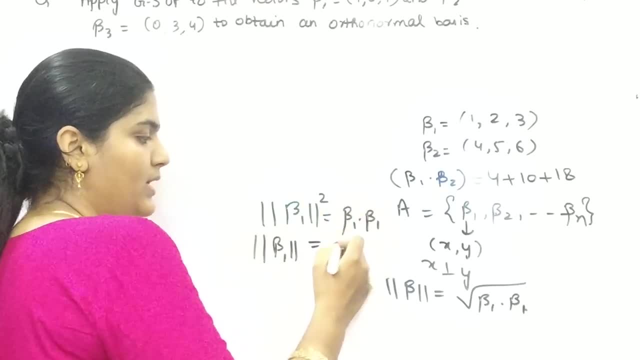 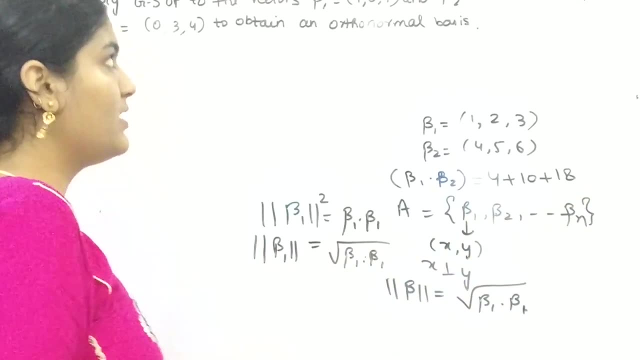 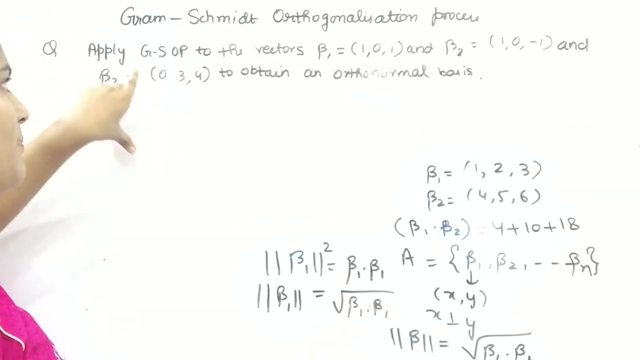 if you want to find out only one number, then that will be square root, Isn't it? And you know how to find this with this form. So let's begin with a question. This is Gram-Smith Orthogonalization process. What you can do for this. You need to apply and 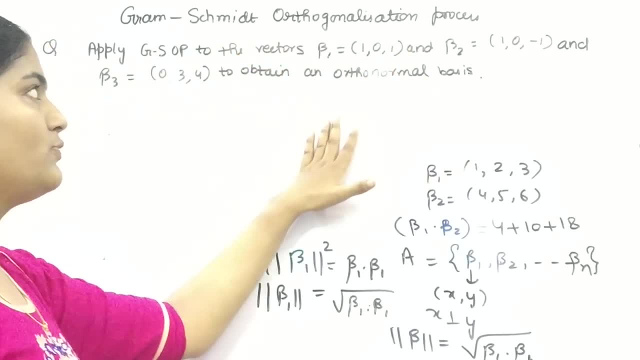 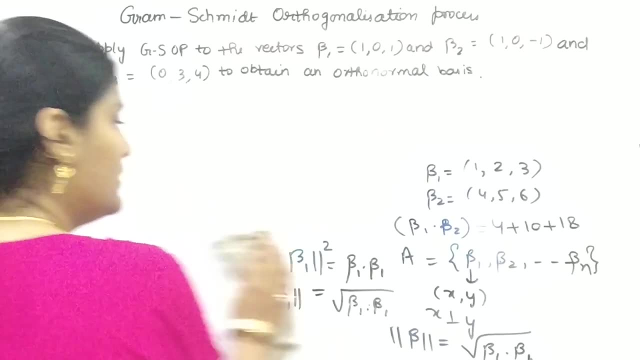 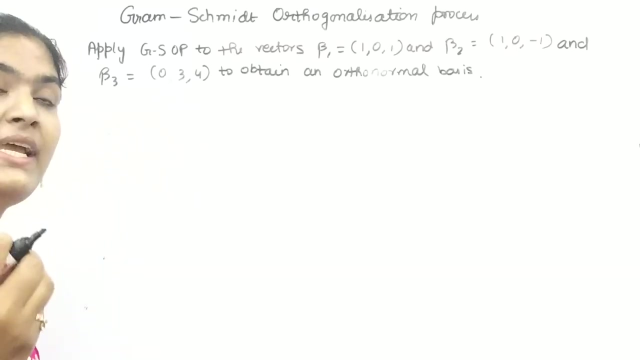 vectors are given to you- Beta 1,, beta 2,, beta 3- and you need to form orthonormal bases for inner product vectors. Okay, So let's begin What we can do. Let me grab a dust up. So first of all, as I told you, let me explain you how you can form the 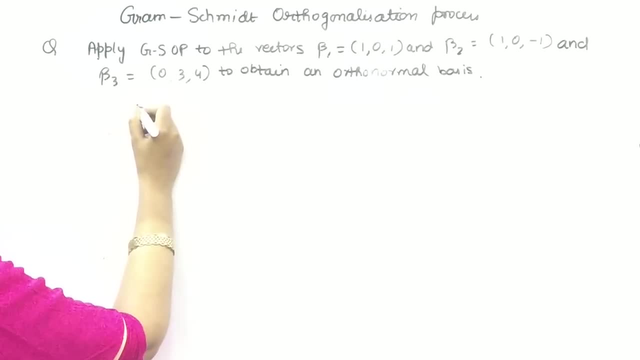 orthonormal bases. Let's say you have any set and your bases for that vector space are beta 1, beta 2 and beta n And your orthonormal bases are alpha 1, alpha 2 for every respective value. Okay, This is your orthonormal bases. 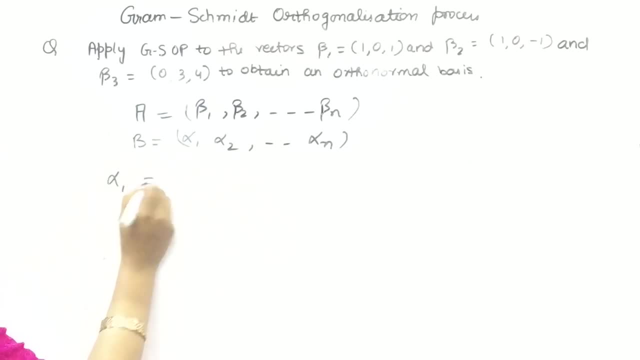 So how you can find them. For alpha 1, you need to do beta 1,, beta 2,, beta 3,, beta 4,, beta 5,, beta 6,, beta 7, beta 8,, beta 9,, beta 10,, beta 11,, beta 12,, beta 12,, beta 13, beta. 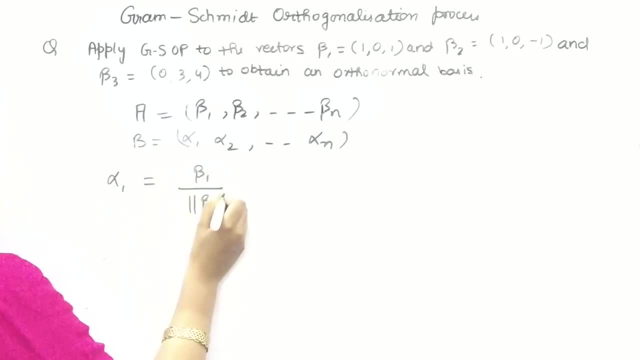 13,, beta 14,, beta 12, beta 14,, beta 15, beta 12 and beta 13.. For alpha 1, you need to do beta 1 and divide it by its base. Okay, For alpha 2, you need to do gamma 2 and divide. 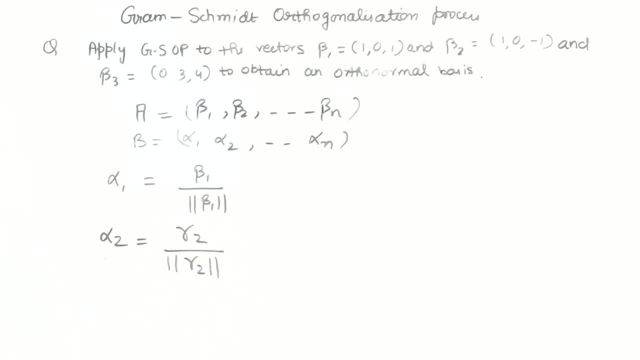 it by its base, Its mode: Alpha 3, gamma 3, divide by its mode. Now you might be wondering what are these gamma and all how they came up, because you have gone through beta 1 and alpha 1.. and all those so on, but not gamma 2.. 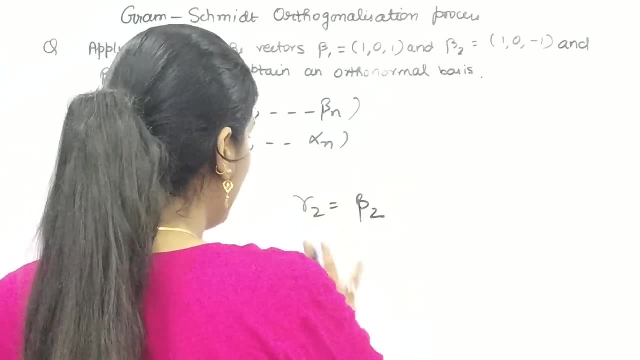 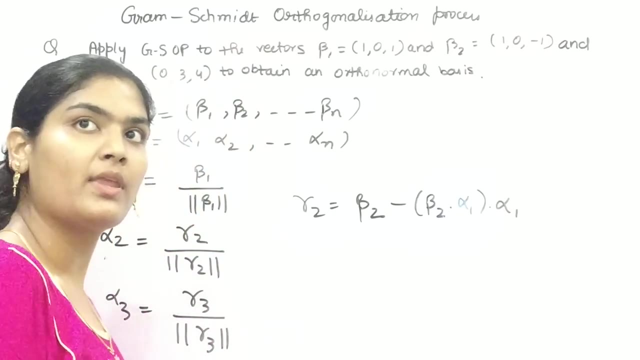 So for the value of gamma 2, how you can find it, you need to take beta 2 minus inner product of beta 2 and alpha 1 with alpha 1.. So beta 2 and inner product of beta 2, alpha 1 and that product with alpha 1.. 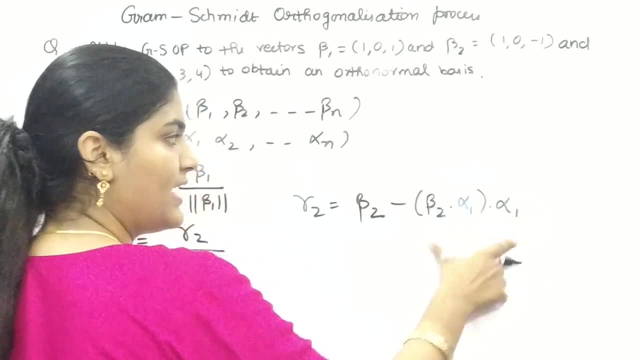 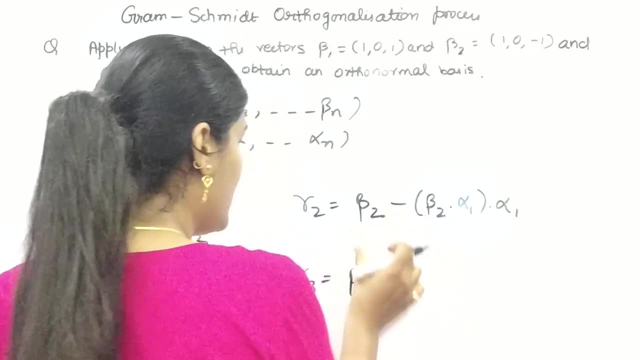 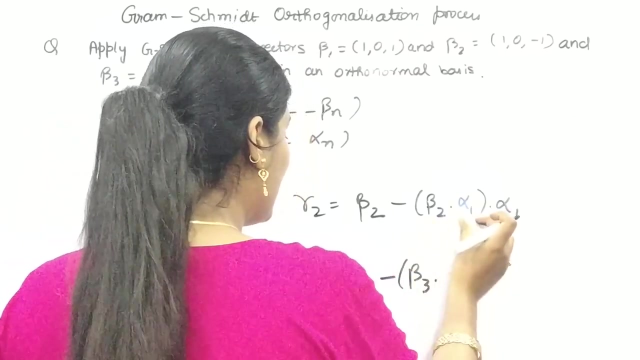 This is inner product and this is simple product where you will get a vector space. Similarly, when you will do gamma 3, it will be beta 3 minus. you can imagine: this is beta 3, thereafter beta 3 dot, this is beta 2 alpha 1, here beta 3 alpha 1 with alpha 1. 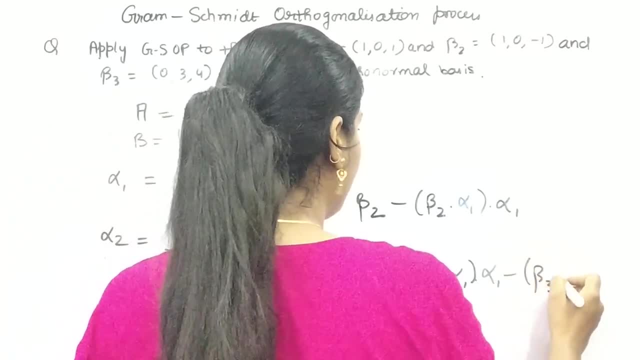 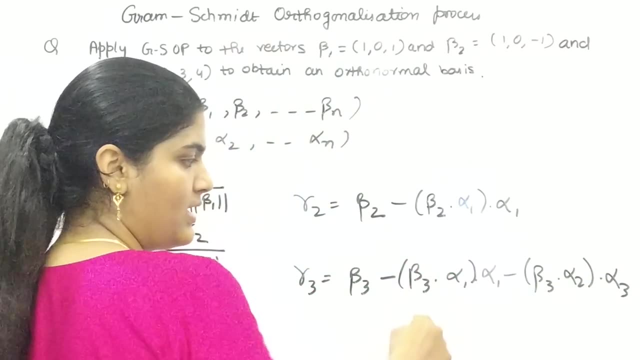 and thereafter beta 3 with alpha 2 as well. Similarly, when you will do gamma 4, it will be beta 4 minus beta 4 with alpha 1, and then you will get beta 3 with alpha 2 as well. 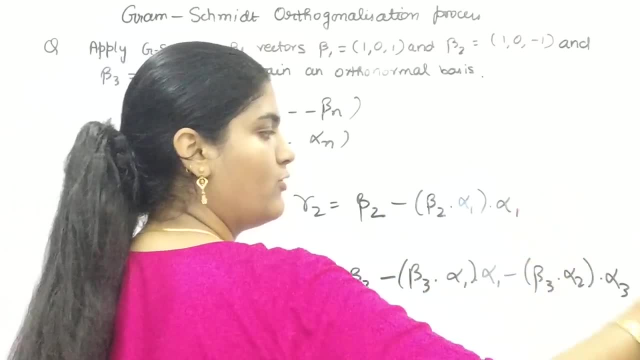 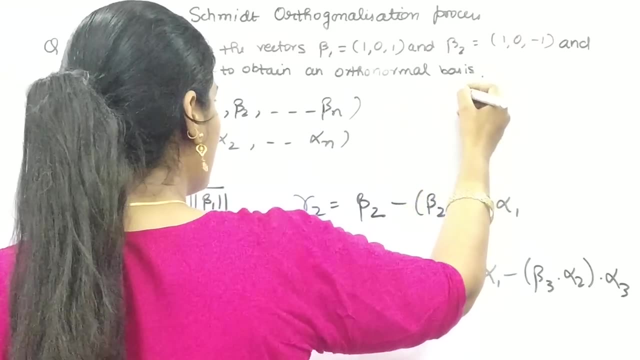 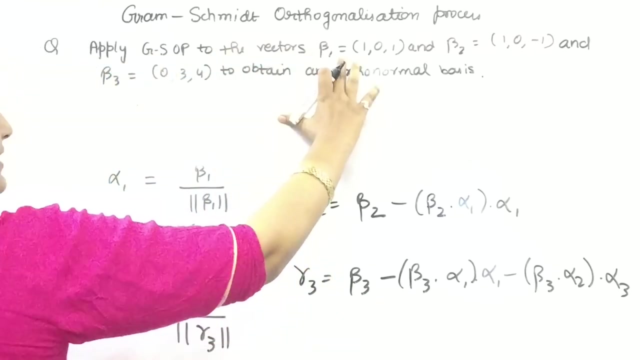 Beta 2, beta 4 with alpha 2, beta 4 with alpha 3 as well. okay, So let's begin. this is just a formula. Let me write it here so that you can. okay, Now you can see. these are your beta 1,. 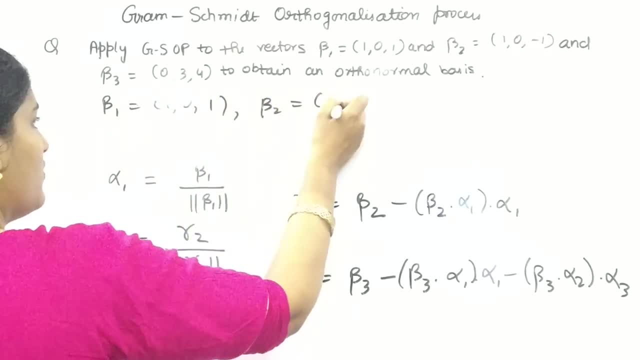 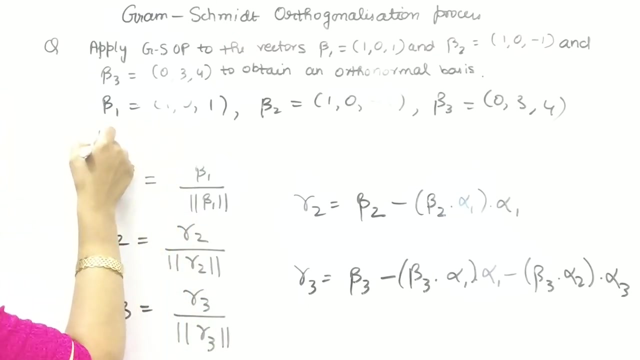 1, 0, 1, 1, 0 minus 1 and 0, 3, 4,. right, Let's begin. first orthonormal base, it would be beta 1 by beta 1 mod. We have beta 1, but how we can find out beta 1 mod? 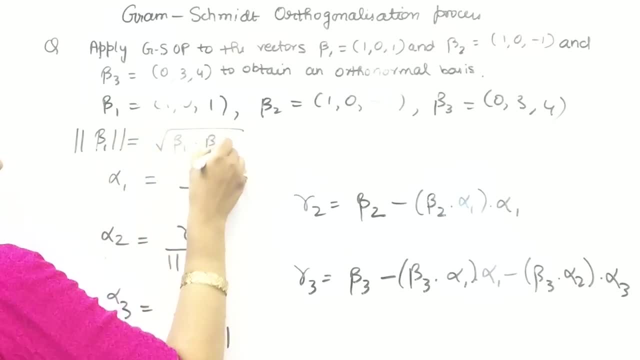 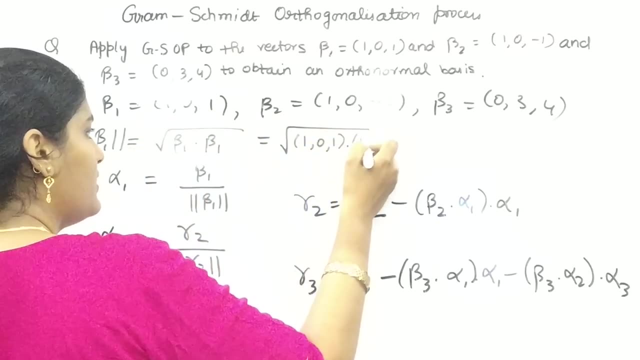 By taking square root of beta 1, inner product of beta 1 and beta 2, right, So this is 1 0 1 dot 1 0 1, so that would be. you know how to do inner product. 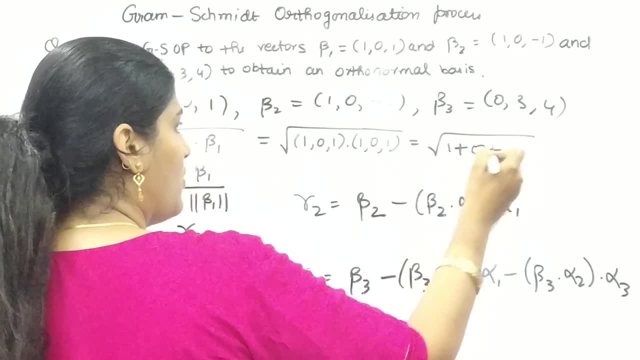 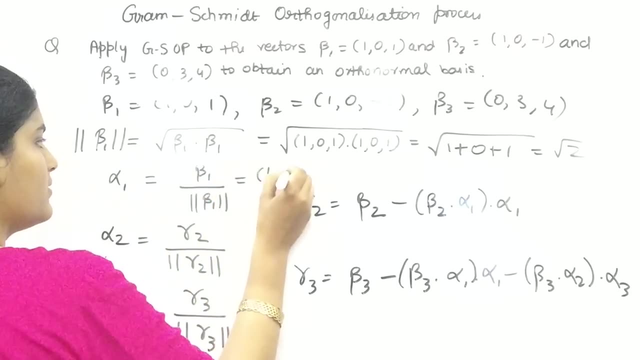 1 times 1, 1, 0 times 0, 0.. 1 times 1, 1, so it would be root 2,. okay, So your alpha 1 is beta 1, which is 1, 0, 1 by mod, which is root 2.. 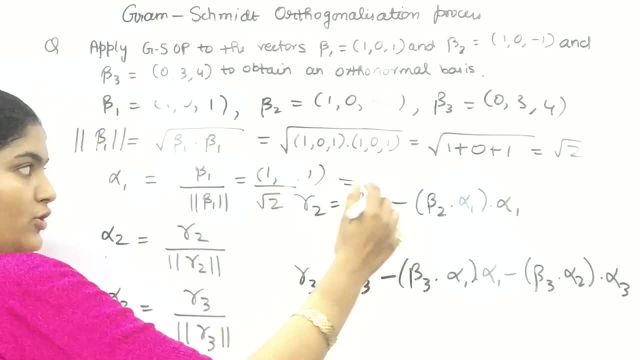 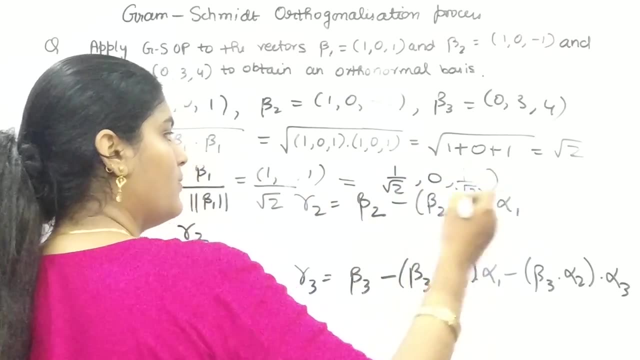 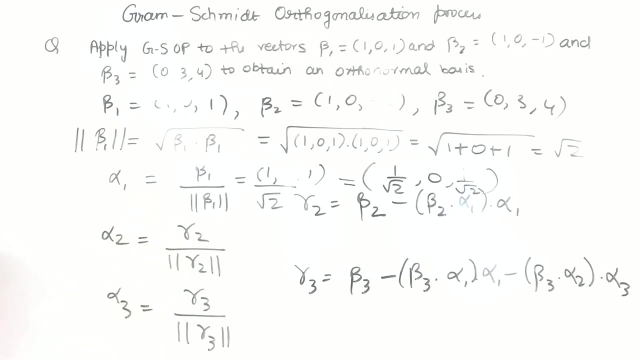 So that means your first orthogonal base is 1 by root 2, 0 by root 2, 1 by root 2, got it Moving on to second orthogonal base. now you need to find out gamma 2. And how you can find the gamma 2 value. 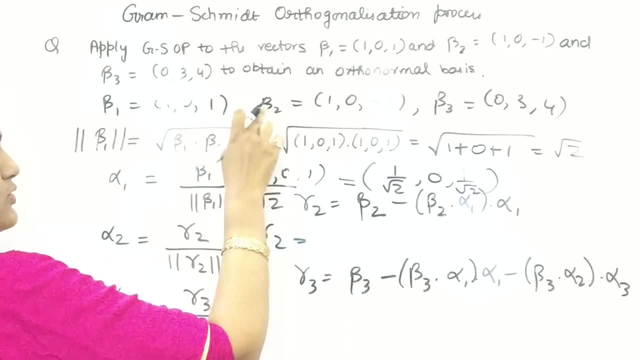 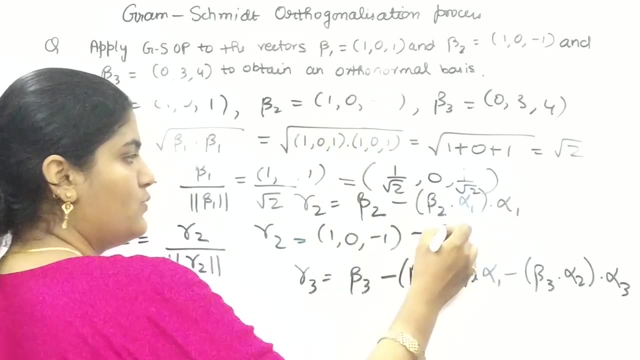 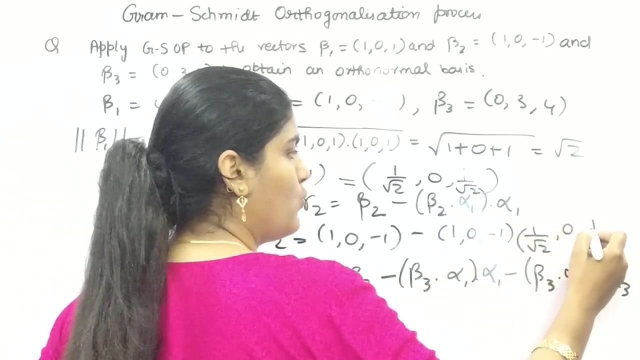 By this. so this is beta 2, beta 2 is 1, 0, minus 1, minus inner product of beta 2, with alpha 1, which is 1 by root 2, 0, 1 by root 2, and with it you need to multiply your alpha 1 again, right? 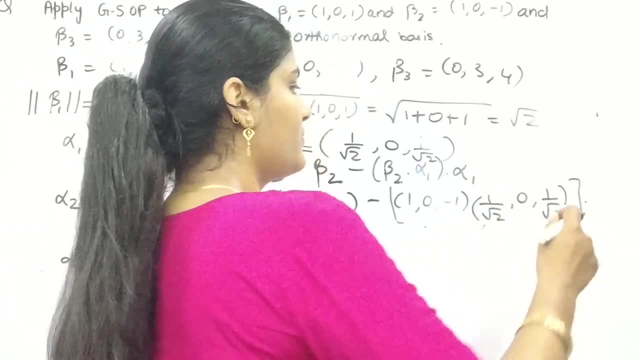 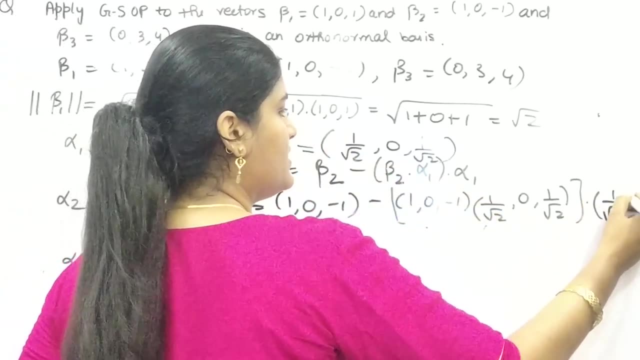 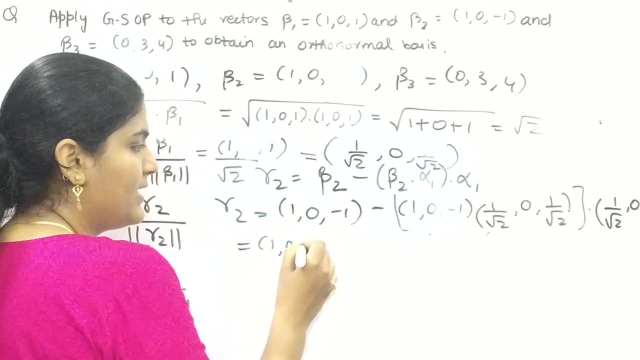 So let me do it Here. so for alpha 1, your value is here 1 by root 2, 0, 1 by root 2, right. So you can see here 1, 0, minus 1, what it would be. 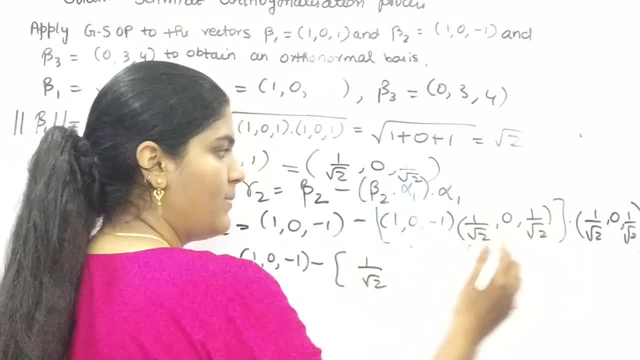 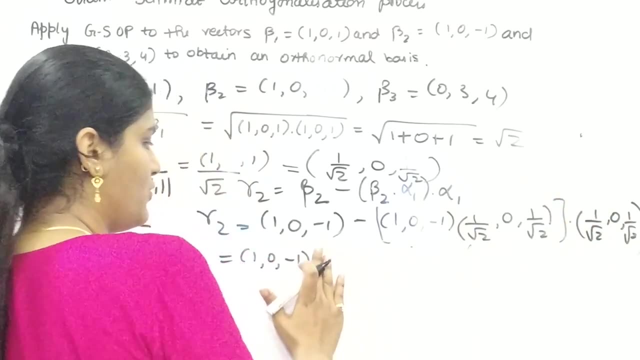 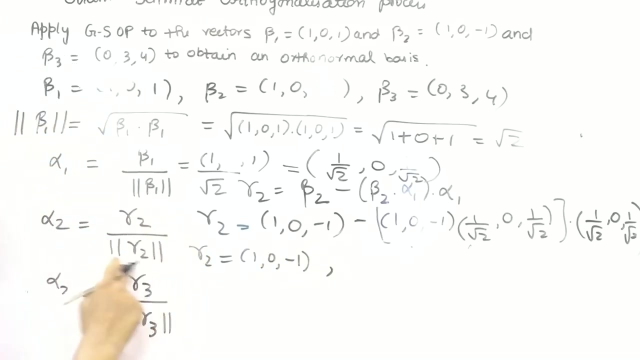 1 by root 2, plus 0, minus 1 by root 2, right, That means 0, 0. multiply this will be 0. So your Gamma 2 is this only, And for this you need to find out mod of gamma 2 as well. 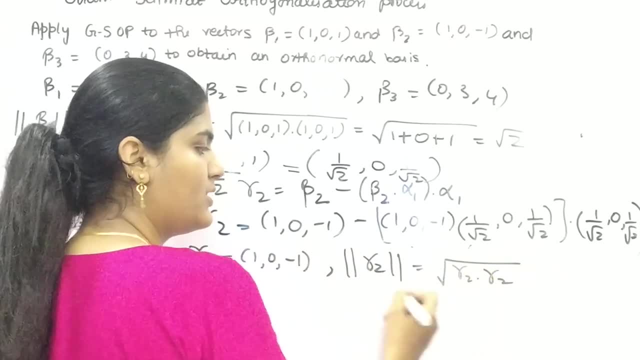 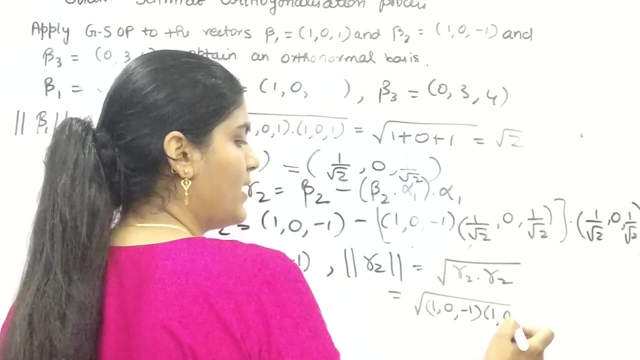 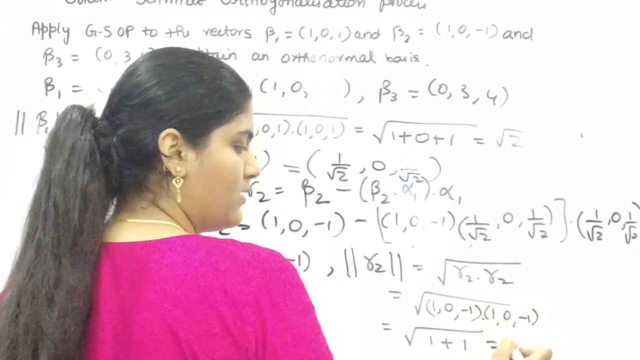 So for that gamma 2, multiply gamma 2, which is your gamma 2, is 1, 0, minus 1, 1, 0, minus 1.. So it would be 1 by 1, 1, minus 1, minus 1, 1,, so root 2.. 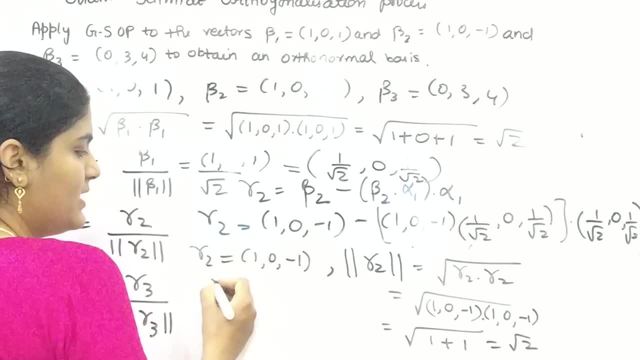 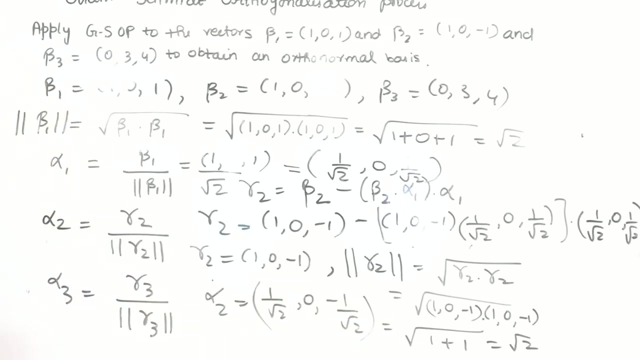 Again, right. So it means your alpha 2 is gamma 2, which is this by this, So 1 by root 2, 0, minus 1 by root 2.. Okay, Then, after what you need to do. third orthogonal space. 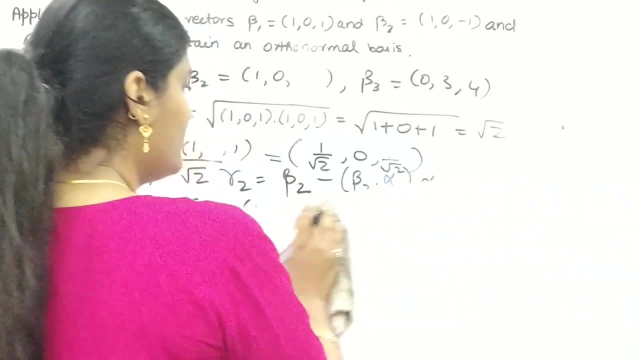 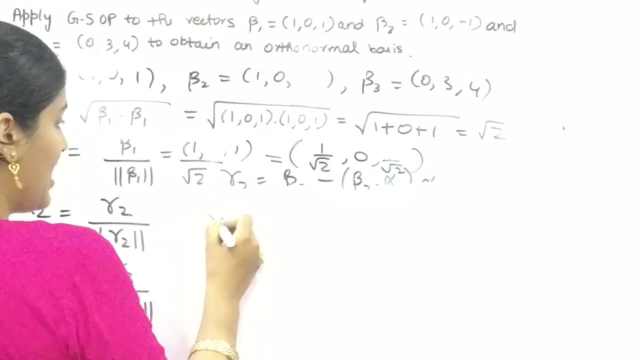 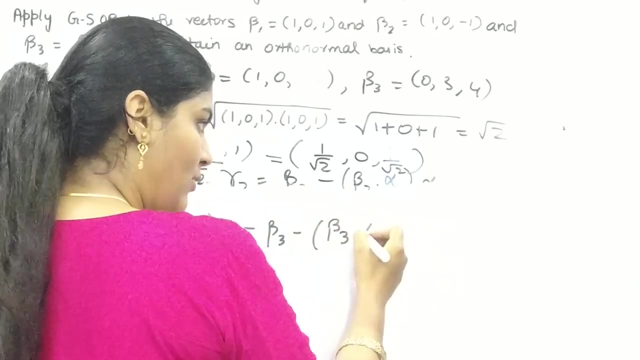 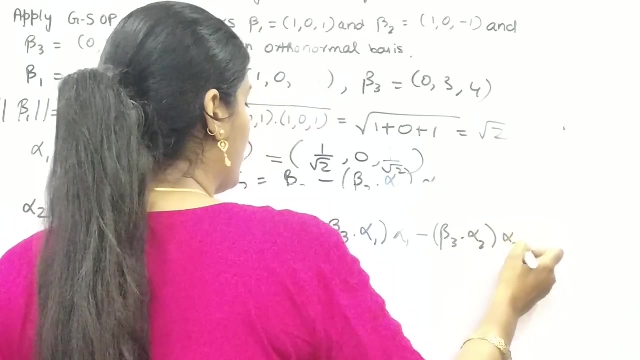 So for third, let me use this. So for third, you need Gamma 3 and gamma 3, well, you, you can compare. you need beta 3, with that, you need beta 3 with alpha 1, right, and then beta 3 with alpha 2, correct. 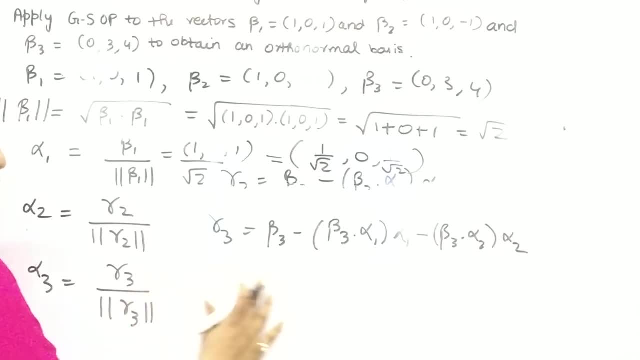 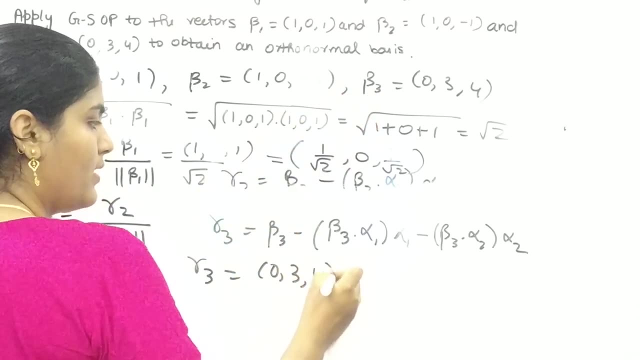 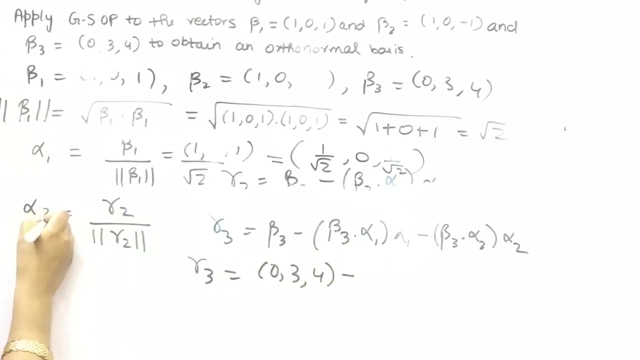 Why, where is our alpha 2?? Oh God, So your gamma 3, your beta 3 is 0, 3, 4, minus. Let me find out. Let me find out it in here. So beta 3, dot alpha 1.. 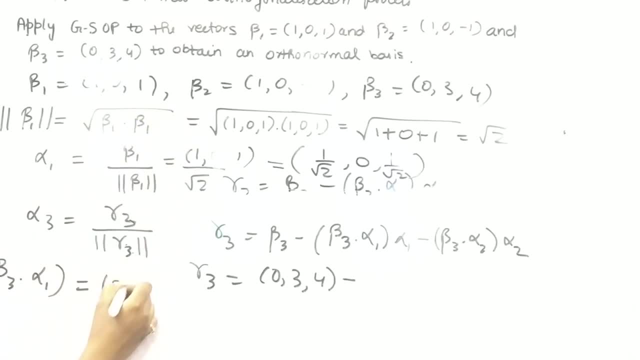 Firstly this: So what is beta 3?? 0,, 3,, 4, and your alpha 1,, your alpha 1, you have already found out here: 1 by root 2,, 0,, 1 by root 2.. 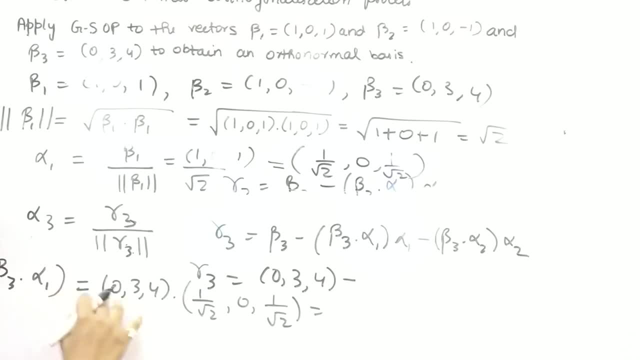 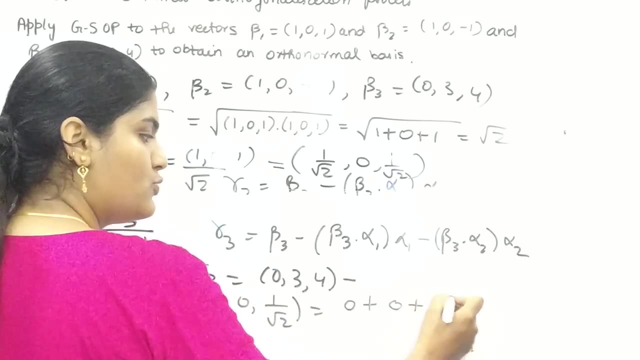 So this would be because it is inner product, inner vector product. so 0, plus 0, minus 0, plus 4 by root 2.. So 4 by root 2 means 2 root 2, right. 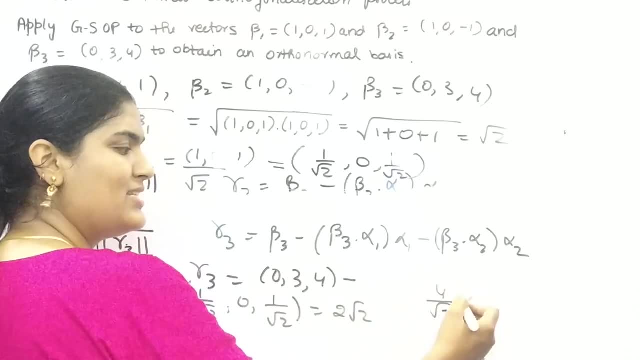 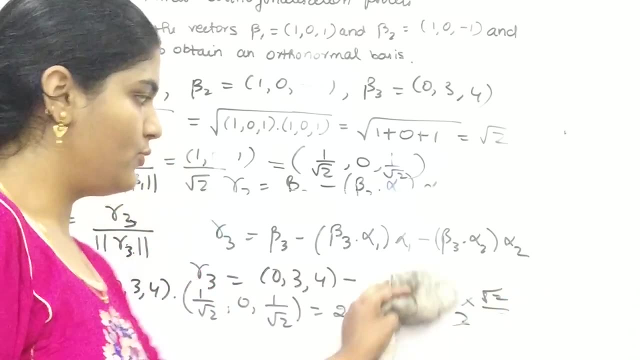 Do you know how to change 4 by root 2 as 2 into? you need to just do rationalization, So 4 root 2 by 2, and this will be 2 root 2.. I know you know it. just to recapitulate. 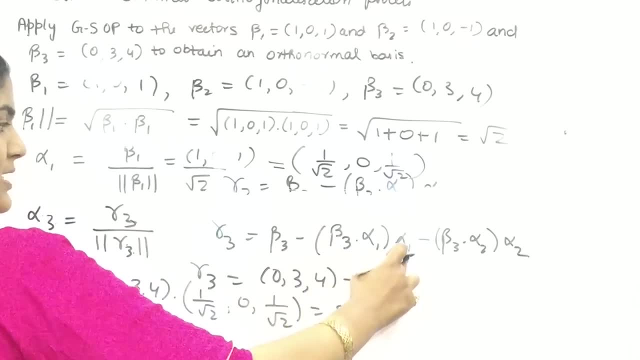 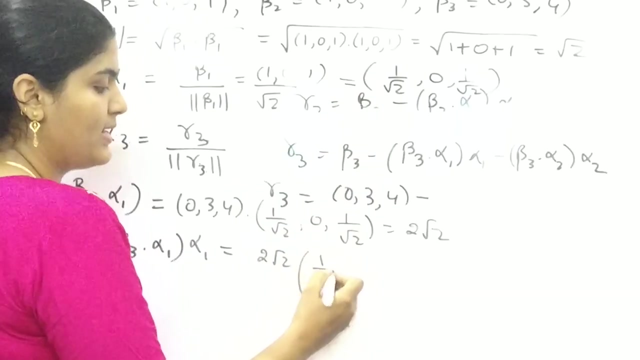 So 2 root 2.. Then after you need to multiply it with alpha 1.. So which is so beta? this value is 2 root 2, but your alpha 1 is 1 by root 2, 0, 1. 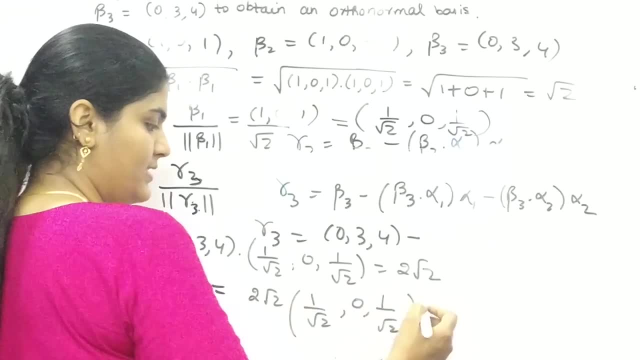 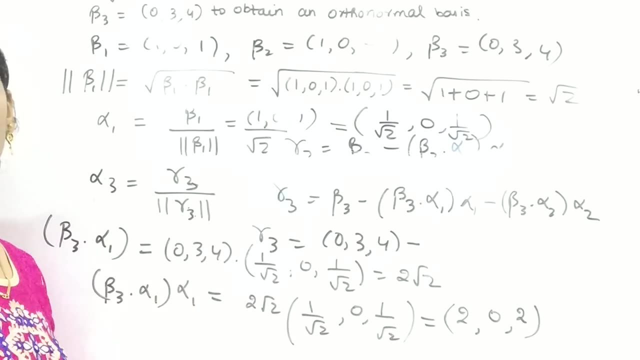 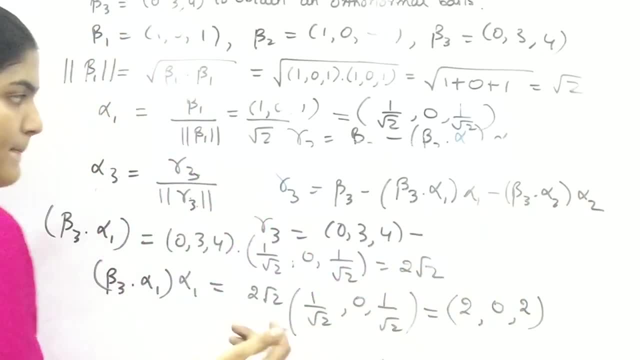 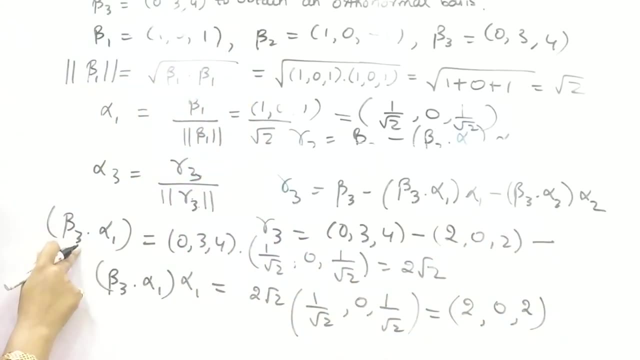 only this value. right Now you need to find this as well. So here you need to put 2, 0,, 2, minus this value. also beta 3 with alpha 2.. Beta 3 with alpha 2.. 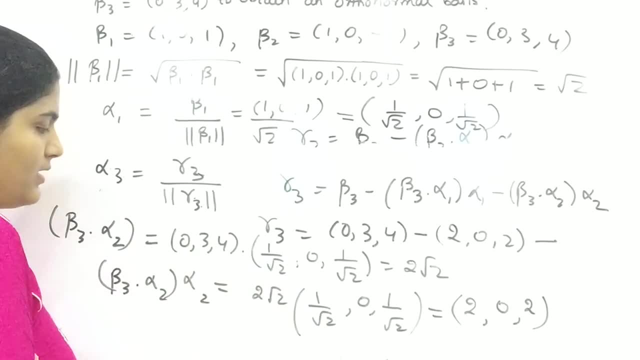 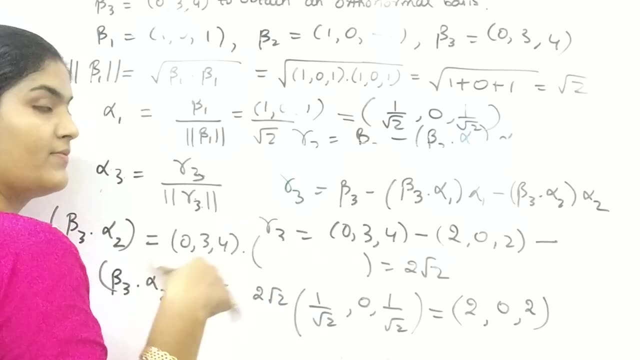 So this is your beta 3.. What was the value of your alpha 2? Because I erased it, so you need to do it. So if you will find out by yourself or you can check the previous one once you will. 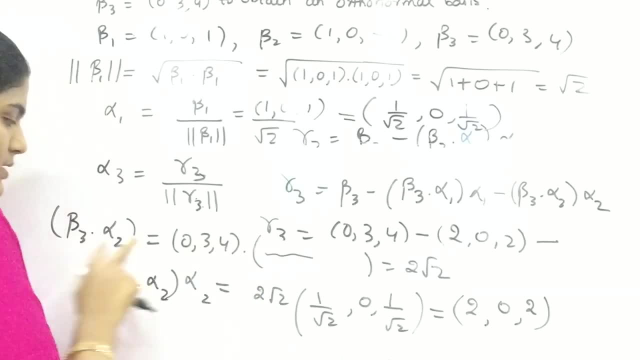 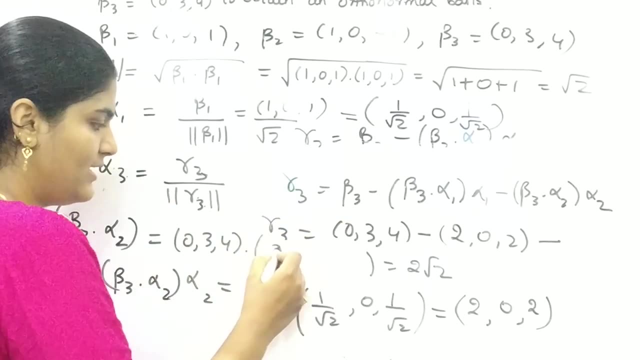 find out the value of alpha 2, put it here. then do inner vector space: 0 multiply first one plus 3 multiply first one. Let's say- I am giving you an example- Let's say its value is x1, y1, z1.. 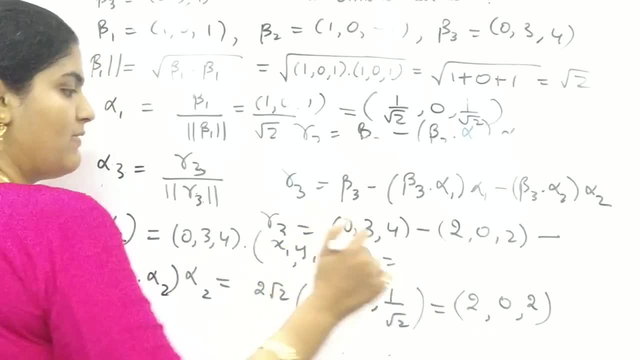 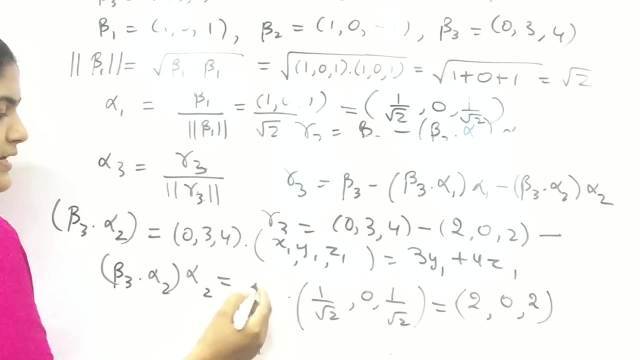 Okay, So 0, x1,, 0,, 3, y1,, 4, z1.. Okay, Thereafter, this is your value: 3, y1, plus 4, z1.. Okay, And you have already.